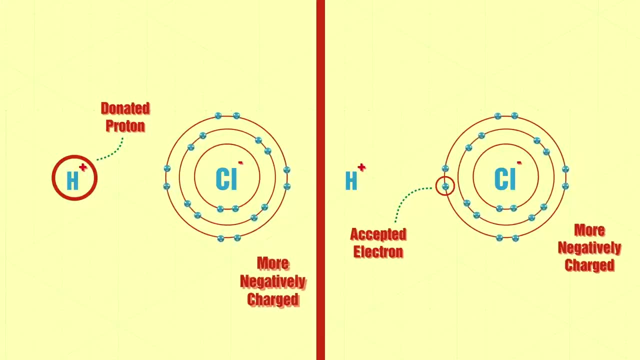 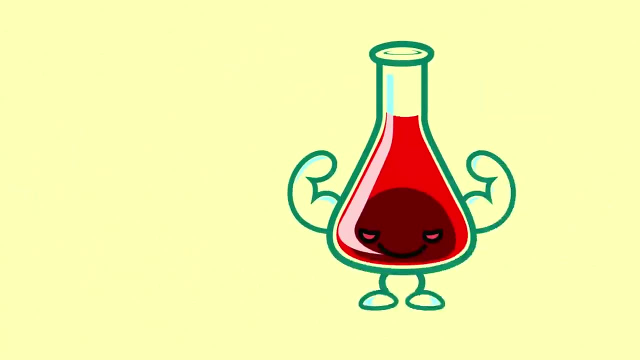 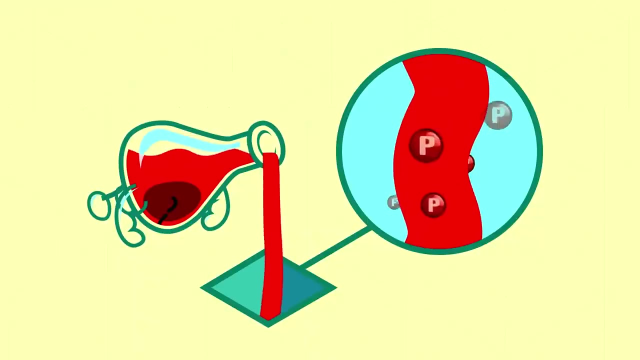 Either way, it's becoming more negatively charged. Other molecules are willing to accept a proton or give up an electron. These are becoming more positively charged. Some substances are so aggressive about donating their protons that when they get a chance, all of the molecules in a sample will dump a proton, sometimes more than one, to the surrounding water molecules. We call these strong acids. What is a strong acid? Meanwhile, some compounds are so ready to accept a proton that they won't wait around. They'll just rip one off water, which usually has two protons but is generous enough to hang out with just one. We call these strong bases. 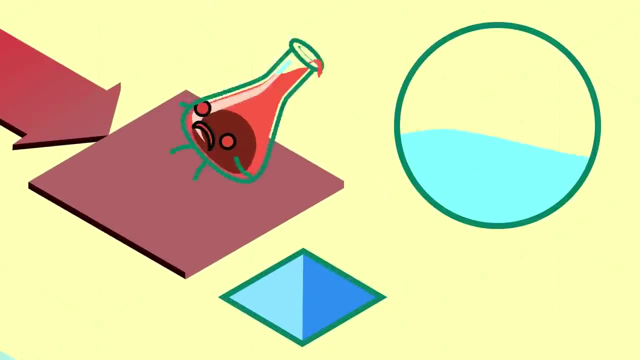 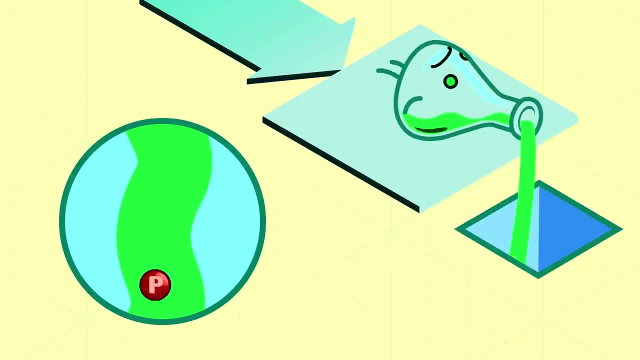 Other acids and bases are not so strong. They may donate just a few of their protons to water, or accept just a few protons from water, but most of their molecules stay exactly the same. 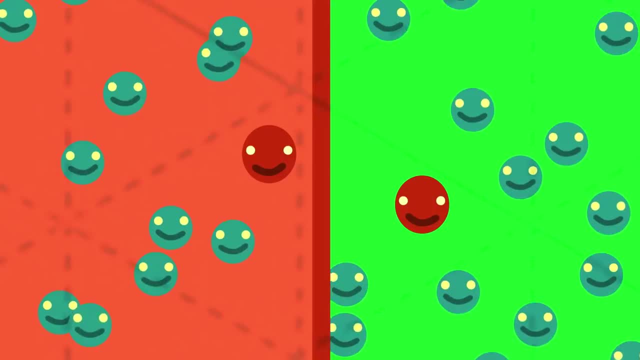 If left alone in water, they'll reach some equilibrium point, where maybe only 1 out of 100, or 1 out of 10,000 of them, will be left alone in the water. 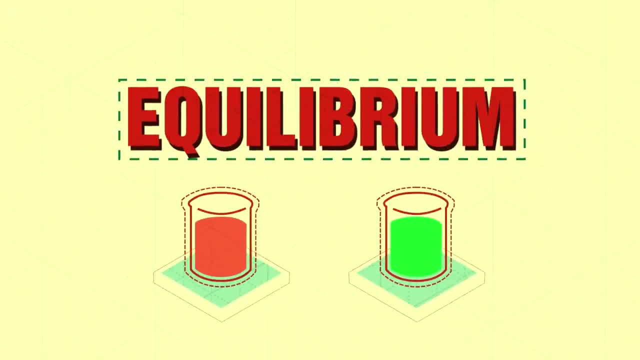 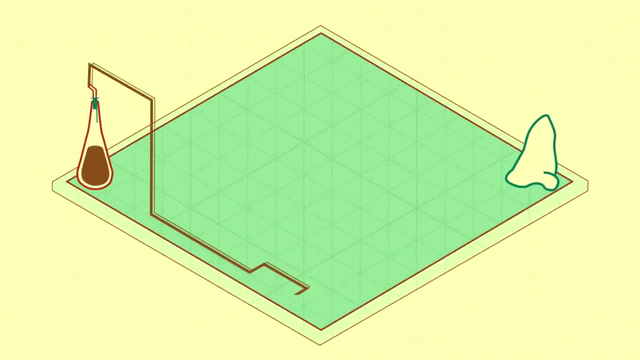 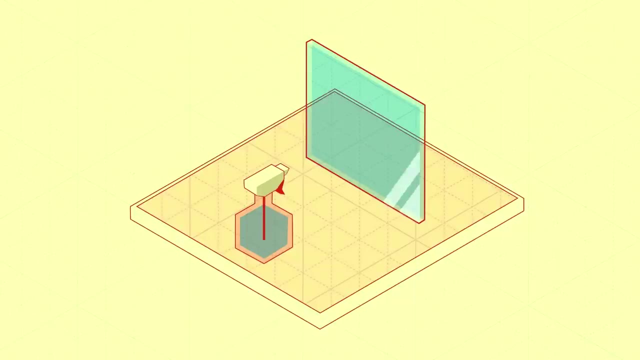 Most of their molecules have exchanged currency with water. As you might guess, we label these acids and bases weak. But in the common sense of the word, they're not weak. The vinegar in your salad dressing that you can smell from across the room? That is a weak acid. The ammonia you spray on glass for a streak-free shine? That is a weak base. 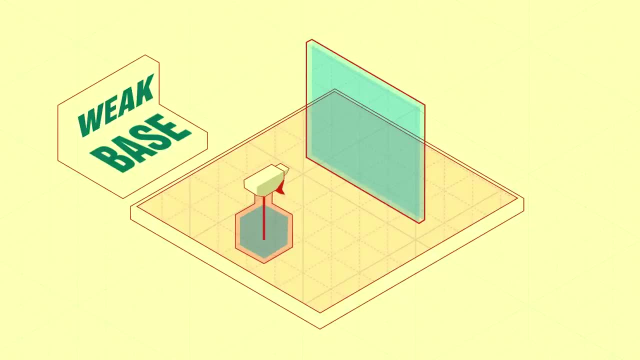 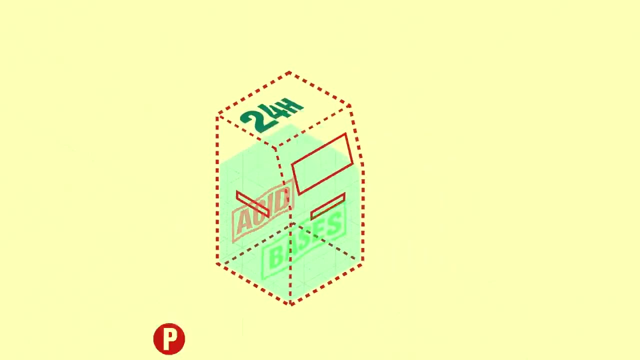 So it doesn't take much to be an active player in the chemical economy. Most acid-base chemistry takes place in water, which can act as either an acid or a base, accepting deposits and enabling withdrawals like a 24-hour molecular ATM. And when a proton deposit customer and a proton withdrawal customer shop at the same time, their net effects on water's account may cancel out. And we call this neutralization. 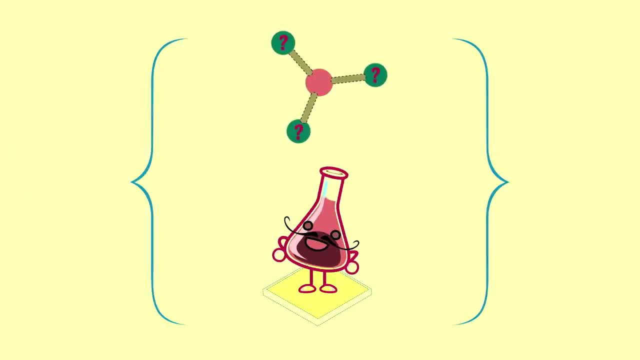 Now certain molecules can behave as acids or bases without water, but that's another story. 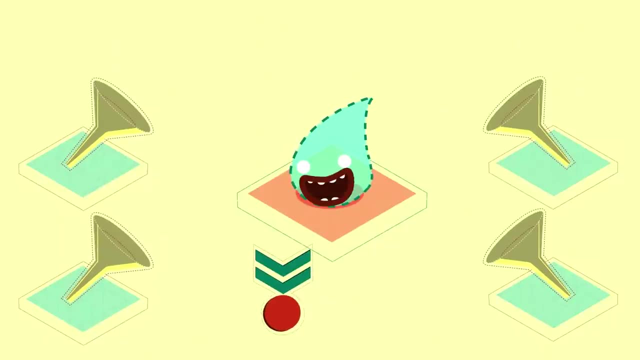 Let's end by saluting water as the resilient and fair banker for acids and bases. It's always open for business, doesn't charge interest, and will never foreclose on your molecules. 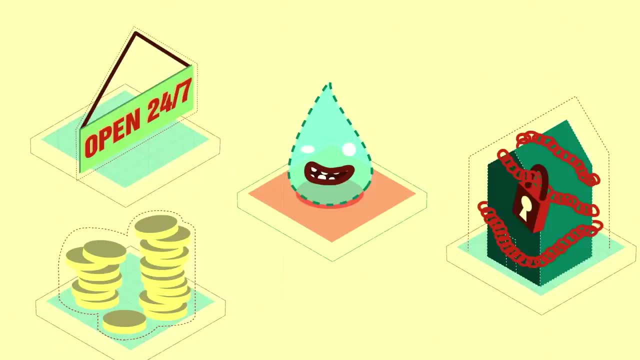 Which is more than I can say for .